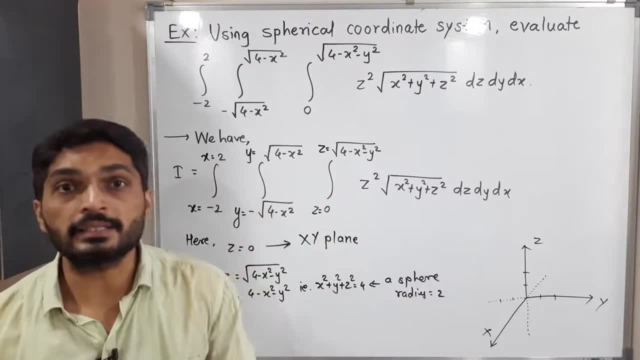 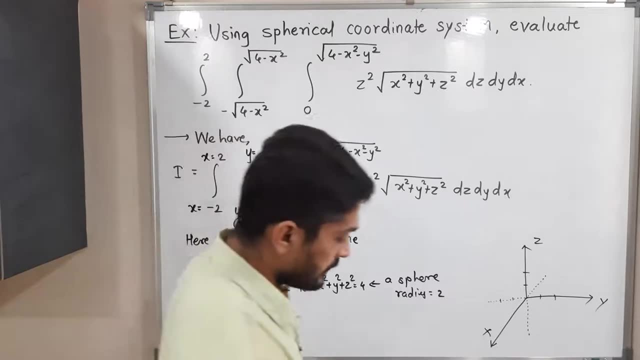 So we should consider upper half of sphere And in any case, if when we have negative square root, that time we have to consider lower half of sphere. So we have upper half of sphere. So let me draw here, I am drawing a sphere: upper half of sphere. So, yes, this. 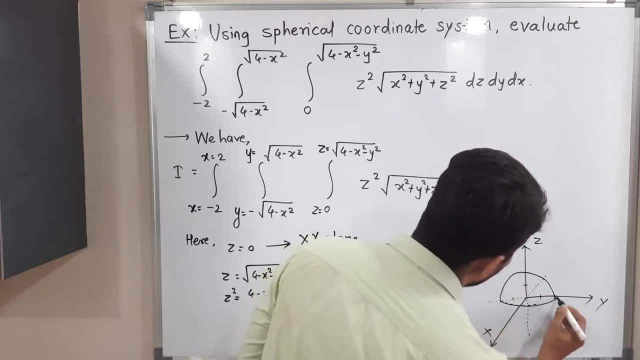 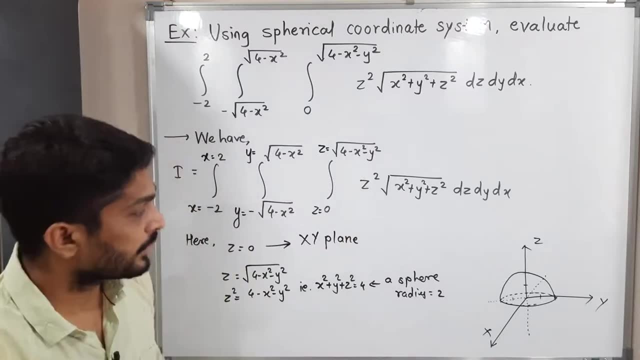 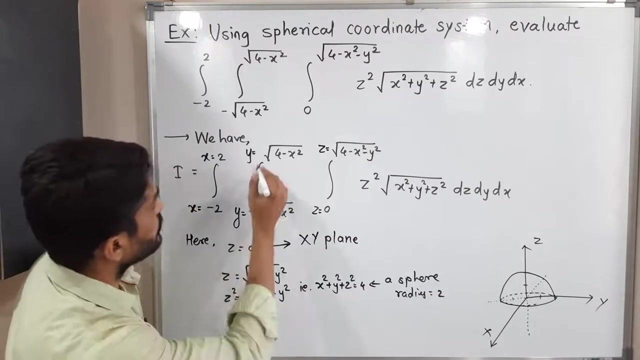 is a sphere we have. Okay, Okay, See, I have drawn a sphere here, upper half of sphere. You can also call it as hemispheres. So radius of that sphere is 2. we have Right, Let us go further. What we have, y is equal to plus minus. Okay, Since we have a limits, plus minus. 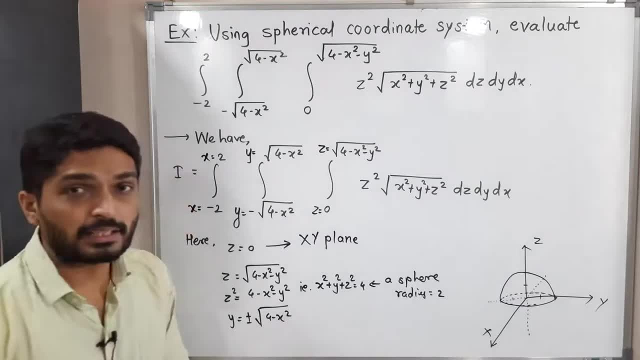 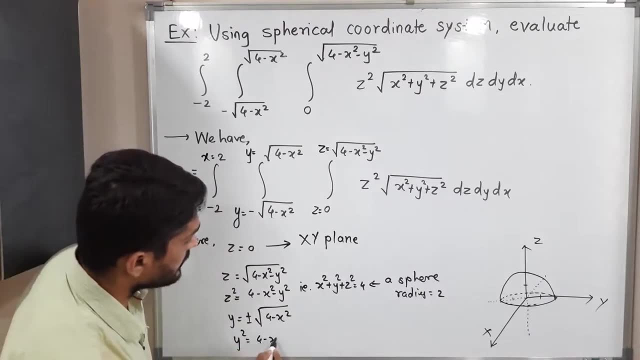 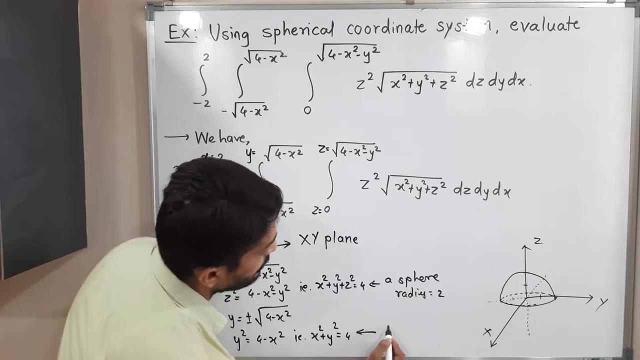 minus square root, of 4 minus x square. The same technique I will use To remove square root. I will take square of both sides, So we will have: y square is equal to 4 minus x square. So that is x square plus y square is equal to 4.. So you know that this is equation. 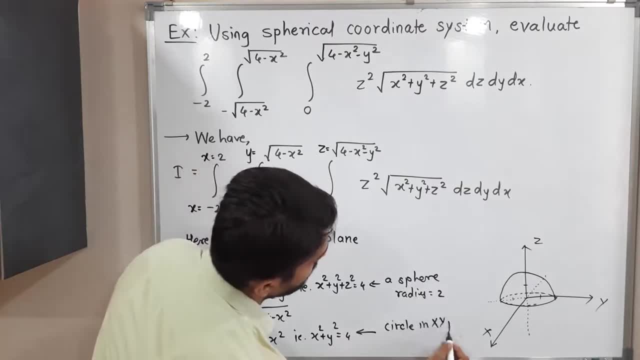 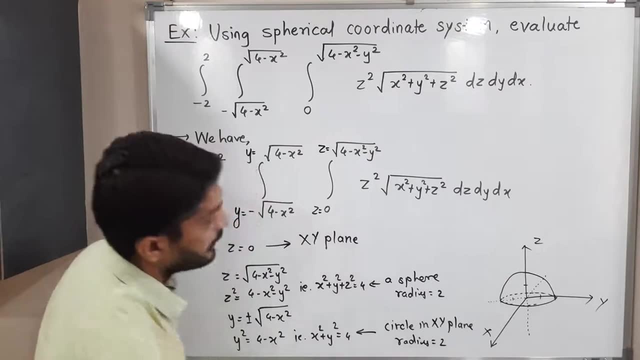 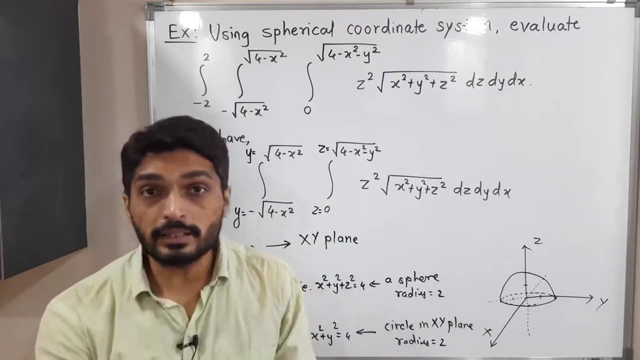 of circle in xy plane. So this is equation of circle in xy plane having radius 2.. So you can easily see here: See in xy plane we are getting a circle. So when the sphere intersects the xy plane we are having a circle. 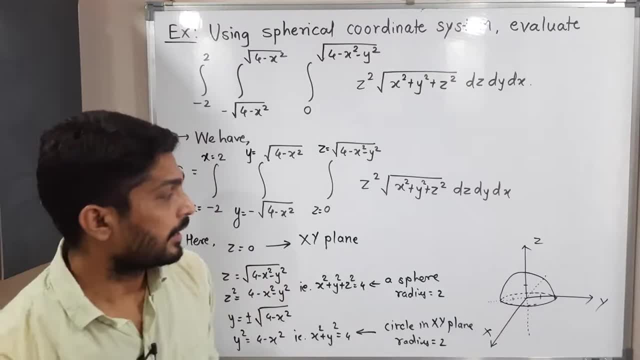 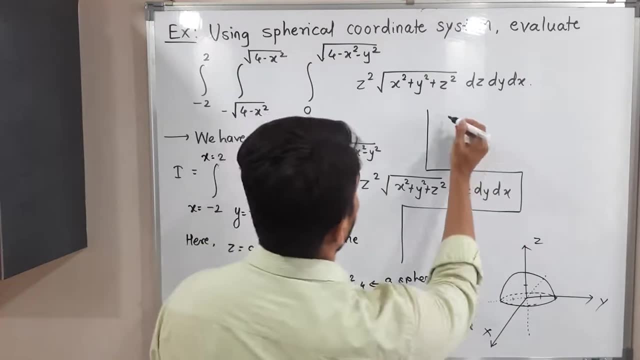 there, with center 0, 0 and radius 2.. After that what we have? x is equal to plus minus 2.. Let me write it here: x is equal to plus minus 2.. x is equal to plus minus 2.. Obviously, here the radius. 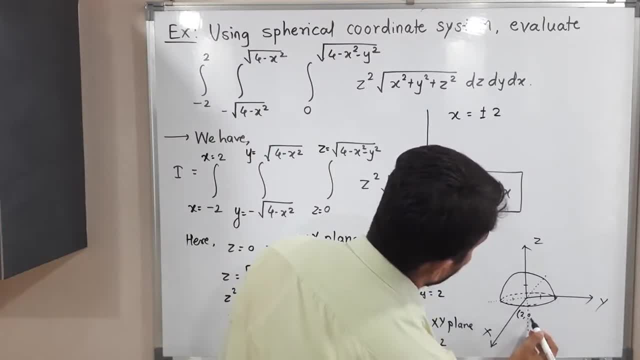 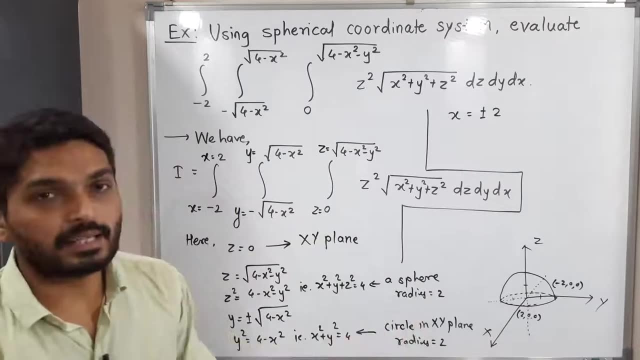 is 2.. So this point will be 2, 0, 0 and on opposite side we will have the point minus 2, 0, 0, right on opposite side. So obviously x varies from minus 2 to 2.. So this thing we have. 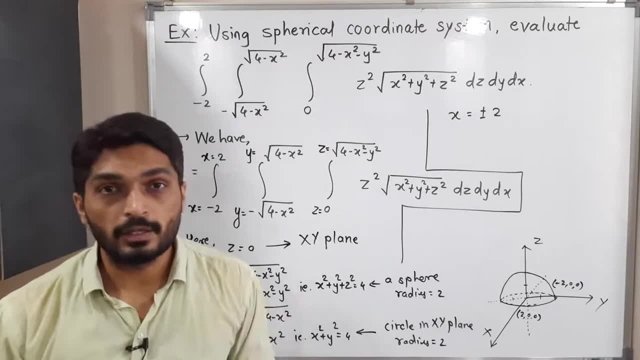 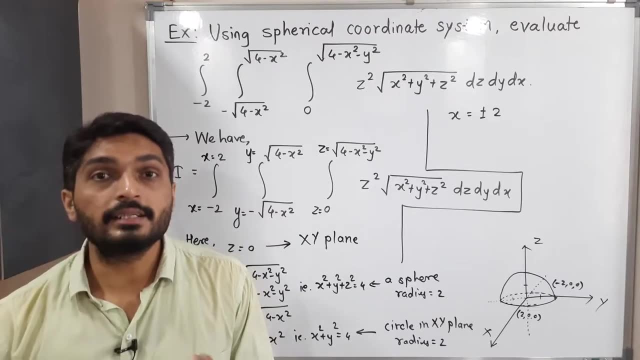 now we have to convert the problem in spherical coordinate system. So for that we have to put: x is equal to rho sine phi cos theta, y is equal to rho sine phi sine theta and z is equal to rho cos phi. We are going to do that thing. Just make a screenshot of it, then we will go further. 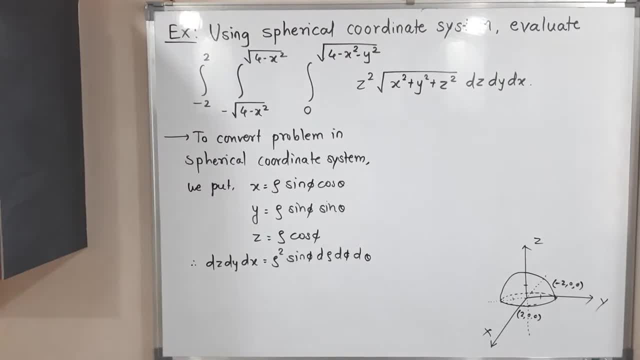 See, and dz dy dx is equal to rho square, sine phi dx d rho d, phi d theta. we have right, See, let us find limits now. Then first we write limits of rho, next phi and next theta, So we have a sphere here having radius 2.. So obviously, 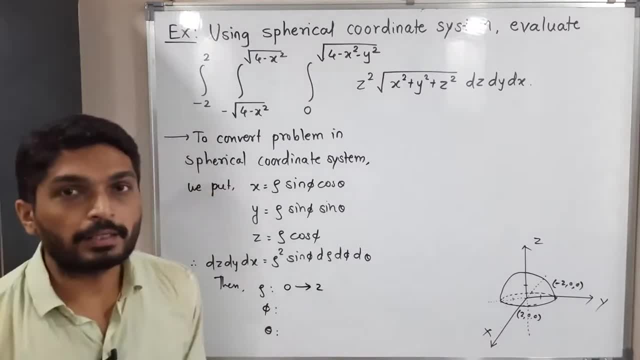 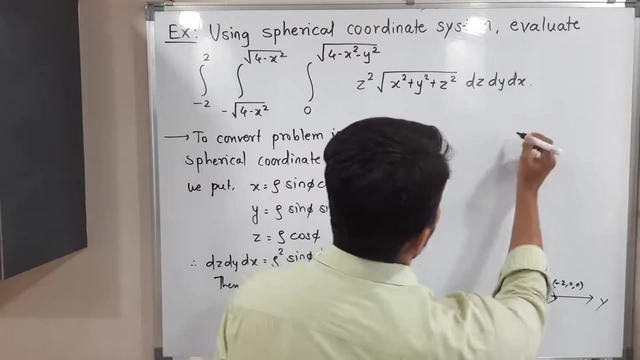 rho will vary from 0 to 2.. After that we have to find limits of phi and theta. We have a upper hemisphere, okay, So I hope still you remember what is phi and theta. in last previous video I have already explained. So when you have point here, 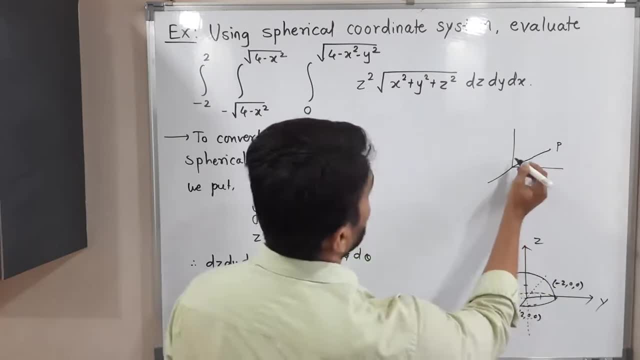 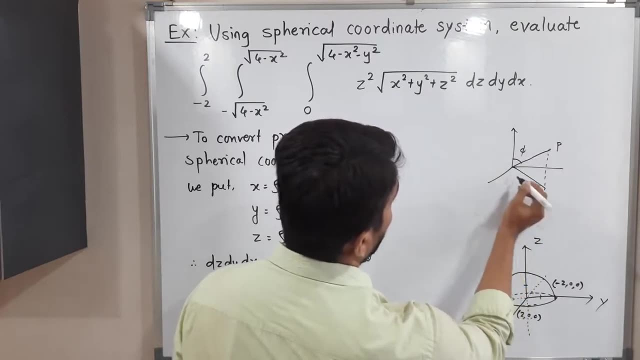 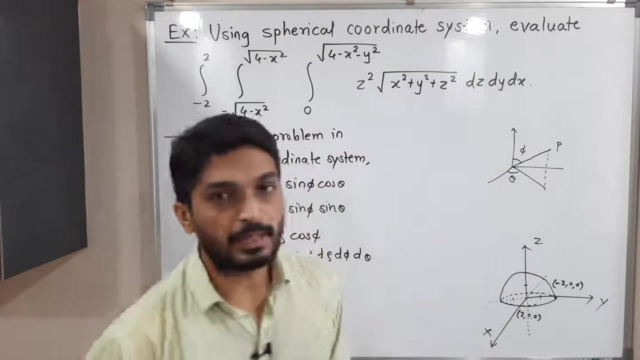 And if you join it to the origin, then it make some angle with positive z axis, that is phi. And when you take its projection on x- y plane, okay, that line makes some angle with positive x axis. that is nothing but theta. So what we have to do, we have to cover this hemisphere. 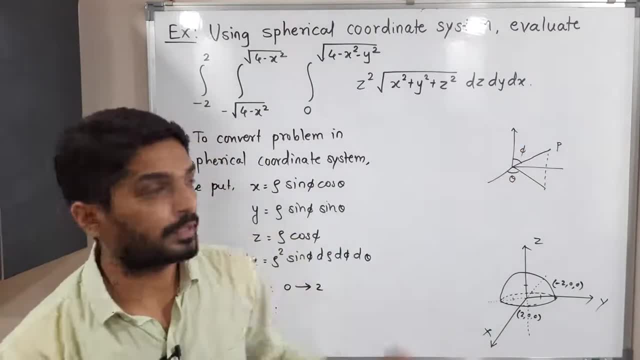 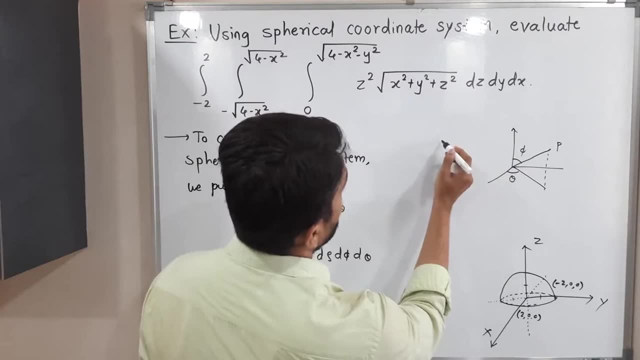 So our phi should be from 0 to pi by 2, getting So 0 to pi by 2, that means we'll have just this part only. Okay, in R3 i am drawing. So, yes, Yes, so we have just 0 to r3, x equal to 0. 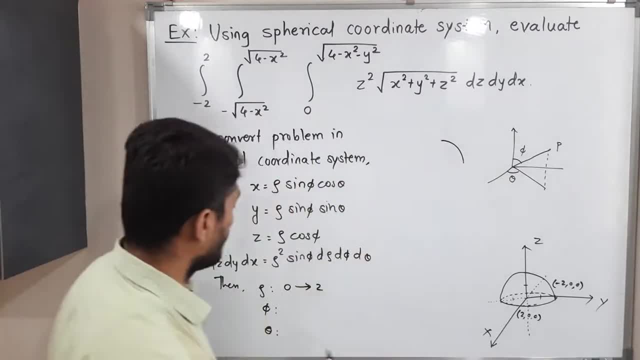 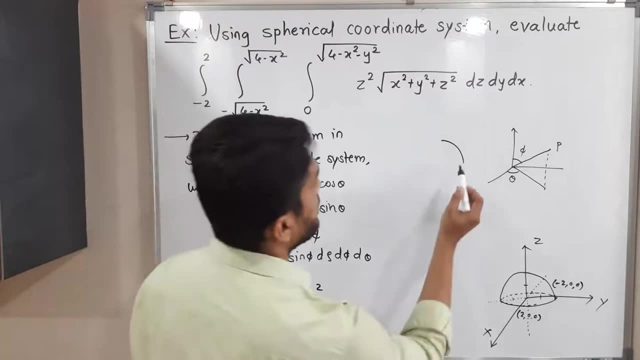 Yes, So we have just 0 to pi by 2,, 90 degree only, So 0 to pi by 2.. And after that, what will I do? Theta? So limits of theta will be 0 to 2 pi, So 360 degree. Okay, This angle theta. So we are. 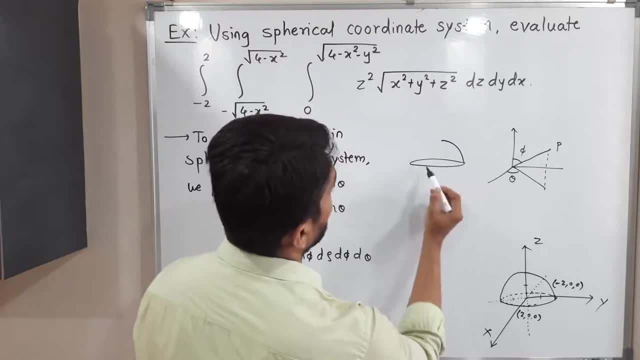 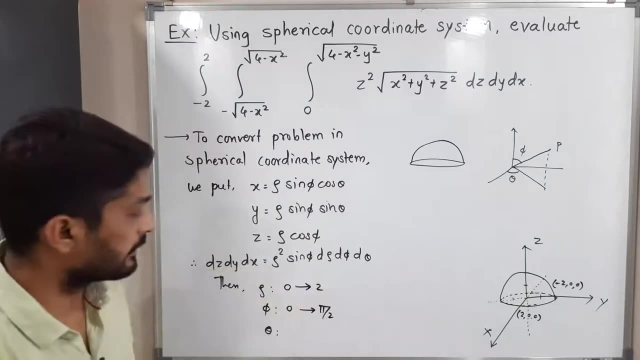 rotating by 360 degree. Okay, So there is a complete circle. So that means if you have this edge and if you rotate by 360 degree, then obviously you will have a hemisphere like this. So in this way we can cover that hemisphere. So theta should be from 0 to 2 pi. Okay. So in this 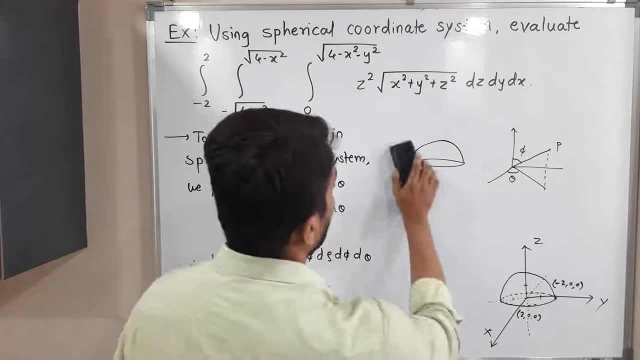 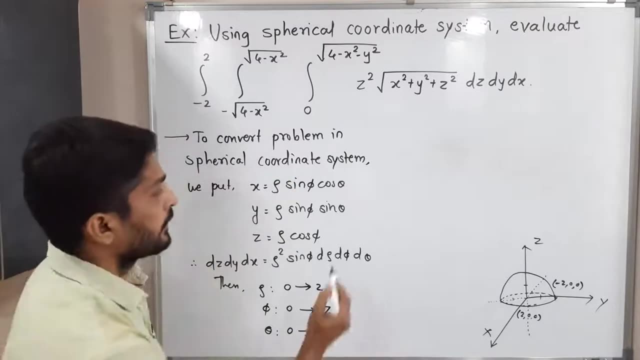 way. we got limits, So let me remove these diagrams. These are not required now. So we have got limits. So simply we have to put, we have to use these new limits in integral and we have to solve the integral. Let us go further. So i is equal to. let me write: Okay, Outer integration. 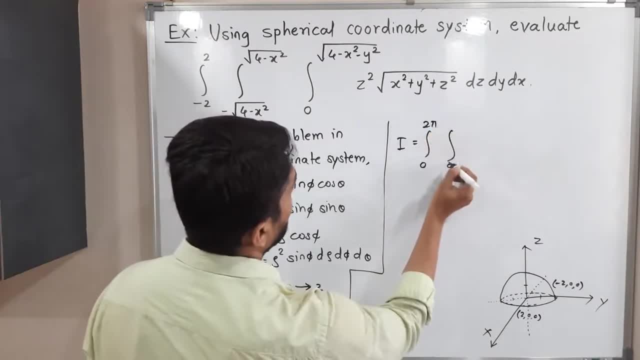 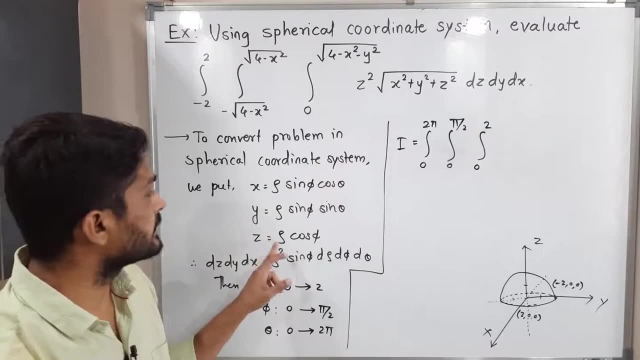 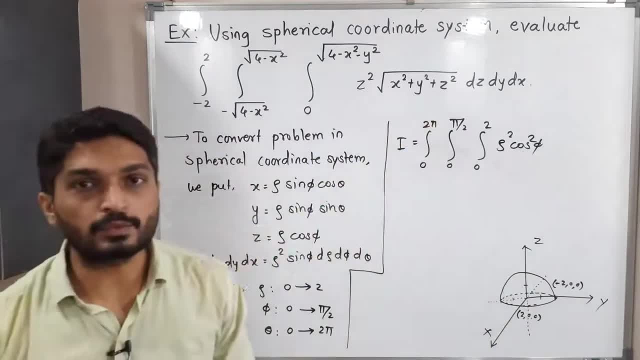 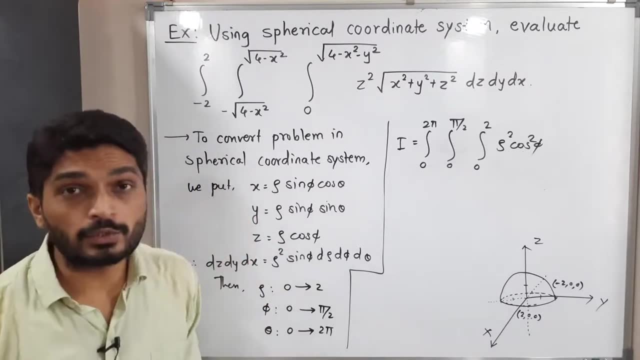 rho square cos phi. So let me write: rho square, cos phi. So let me write rho square cos phi. Next, x square plus y square plus z square. I have already told you in previous video, That is, if I put x is equal to, y is equal to and z is equal to these values, then obviously by solving, 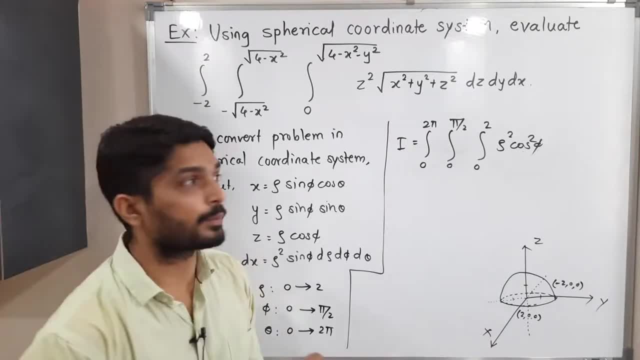 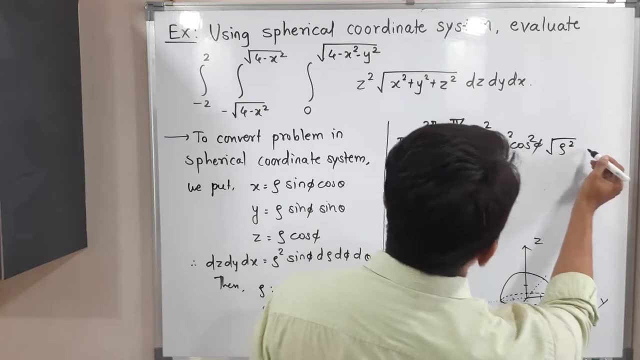 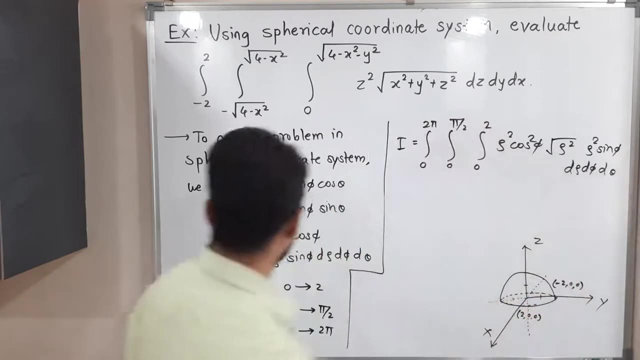 you will have x square plus y square plus z square is equal to rho square. So let me write square root of. what will we have? Rho square right And dz dy dx. That means rho square, sin phi, d, rho d phi and d theta. This thing I have already told you, So let me write square root of: 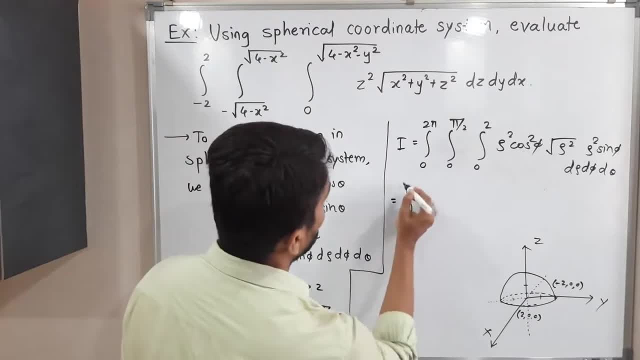 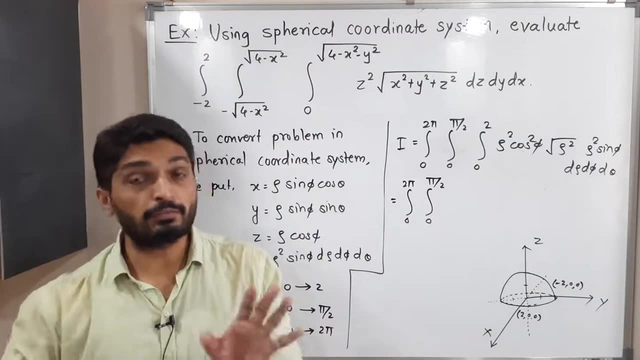 this thing I have already mentioned here. So let us simplify it. Integration 0 to 2 pi. Let us see what will happen. Integration 0 to pi by 2. So only for inner integration rho will be variable when functions of rho and remaining terms will be constants. So I will take them outside, So that 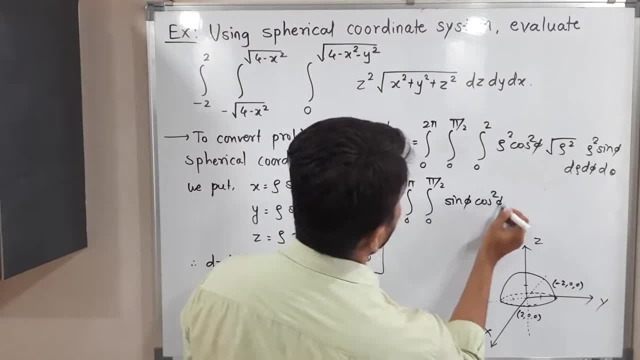 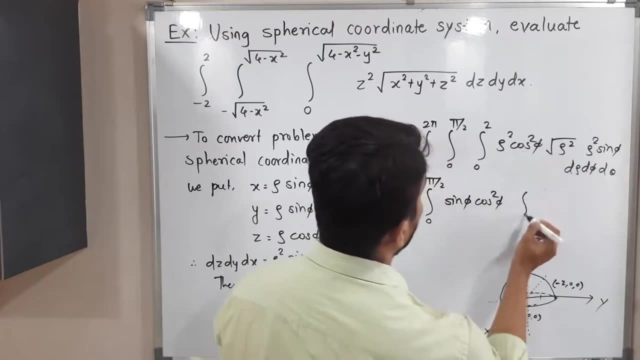 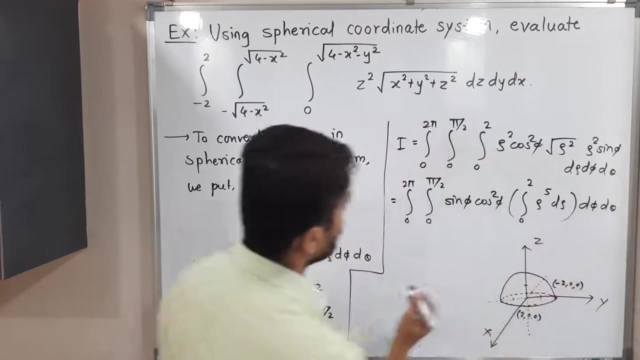 sin phi and cos square phi will be constant. We will come outside. So here square square root cancels. So rho rho square, rho square. That means we will have total rho raise to 5,. 0 to 2, rho raise to 5, d phi, d theta. Let us solve it further. So this is equal to integration: 0 to 2 pi, 0 to pi by 2,. okay. 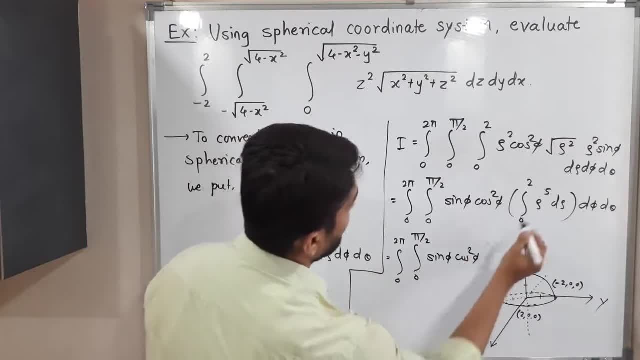 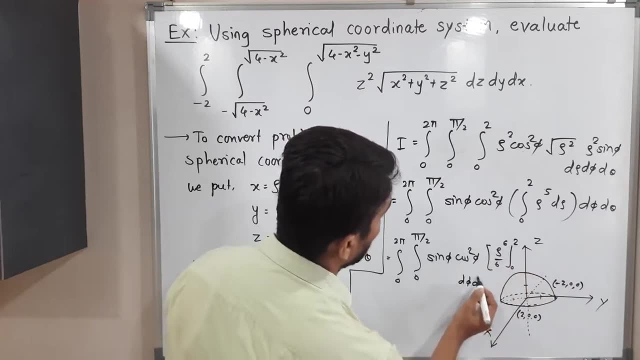 Sin phi cos square phi. Integration of rho raise to 5 is rho raise to 6 by 6, with limit 0 to 2.. I should write here: d rho d d phi d theta. Okay, let us continue. So 2 raise to 6.. That means it will be. 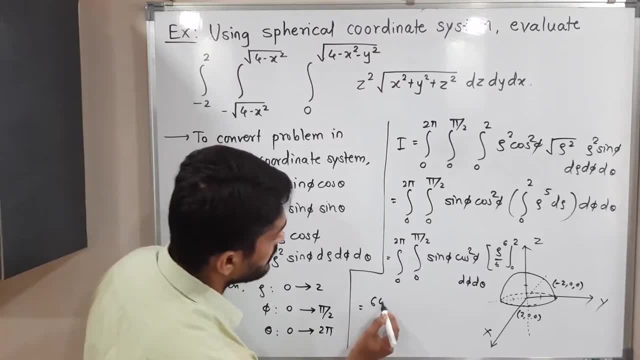 64 by 6.. So it is a constant. We can take it outside: 64 by 6.. Integration 0 to 2 pi. Integration 0 to pi by 2.. Sin phi cos square phi d phi d theta. So now we: 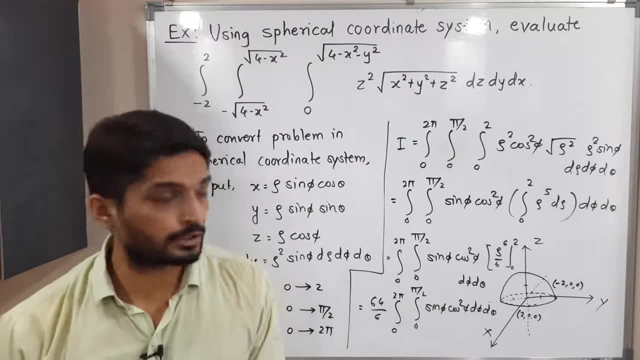 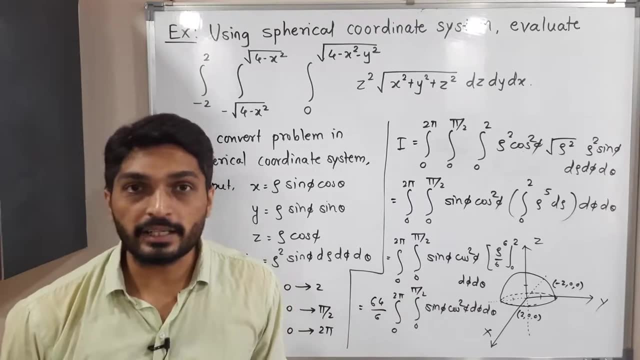 have to integrate with respect to phi. But we have a beta gamma function getting So 0 to pi by 2 limits. we have Sin. some sin raise to something, cos raise to something. That means 101 percent. that definition of beta is applicable here. Make a screenshot of it. After that we will go further. 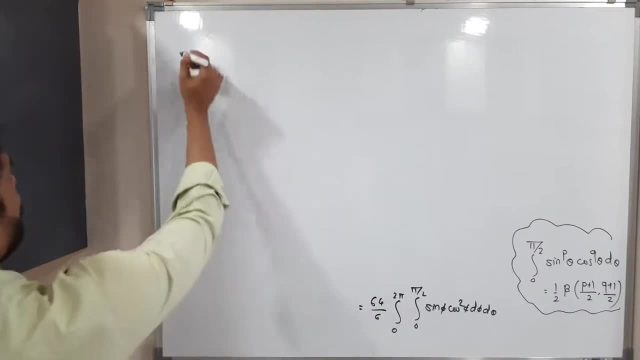 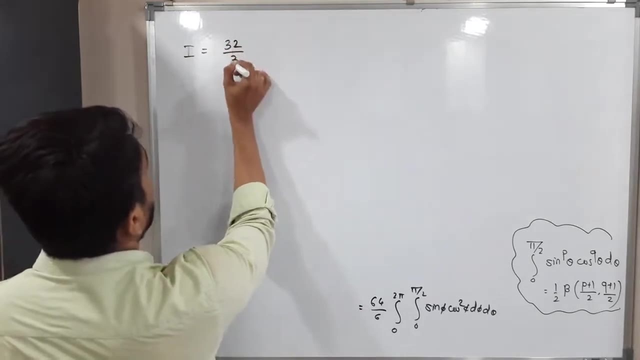 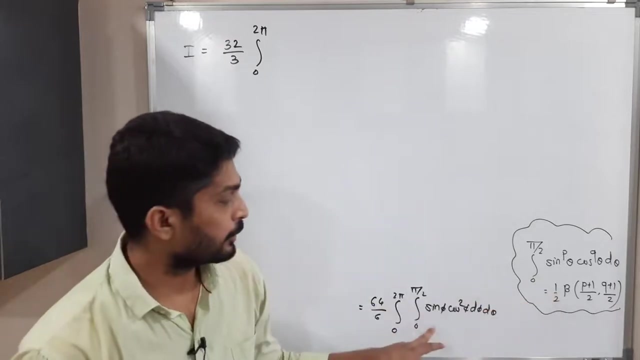 So let us go further. So I is equal to okay. What will happen? That 2, 2 we can cancel here. So we have 32 by 3, okay, Integration 0 to 2 pi. See, I am going to use this. We can convert in beta function. okay, I am going. 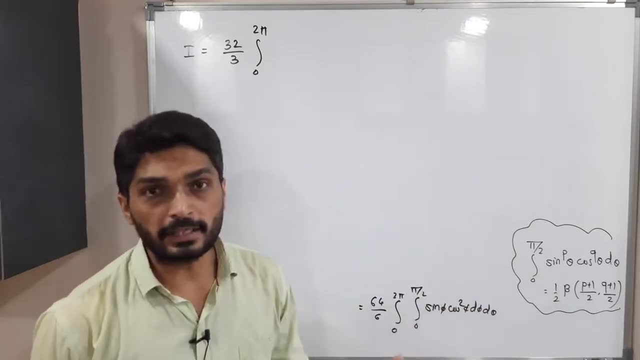 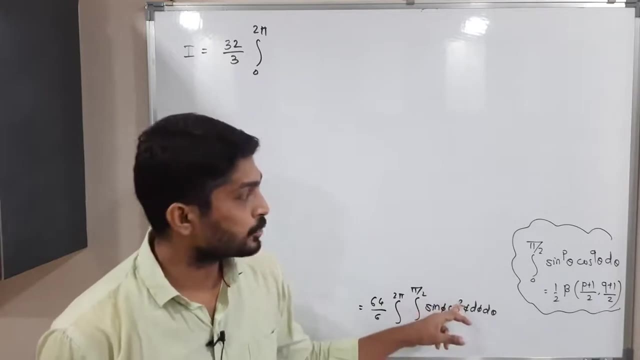 to convert. use this relation to convert it, this integral in beta function 0 to pi by 2, we have right. Sin raise to 1 is there, So value of p is 1.. And cos raise to 2 is there, So value of q is 2.. 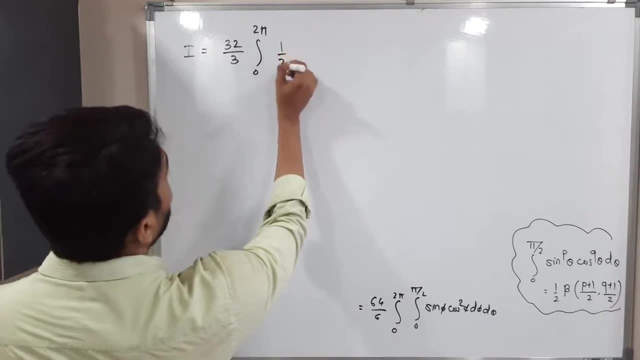 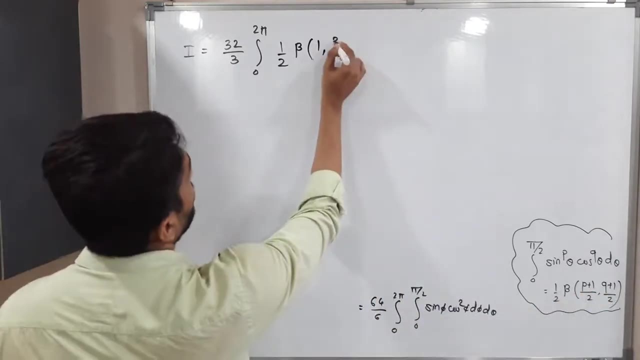 So let us use it. What I should write here: 1 by 2. beta of p is 1, 1 plus 1, 2 by 2, 1.. And q is equal to 2, 2 plus 1, 3 by 2. we will have: 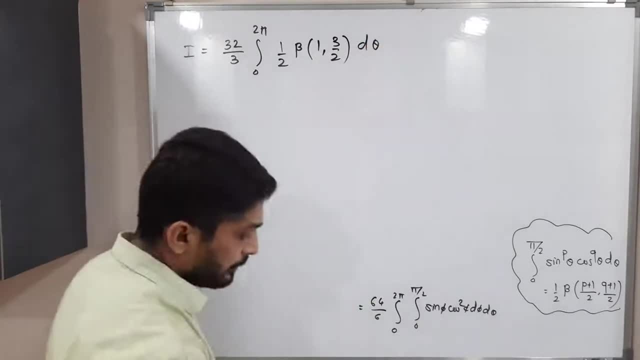 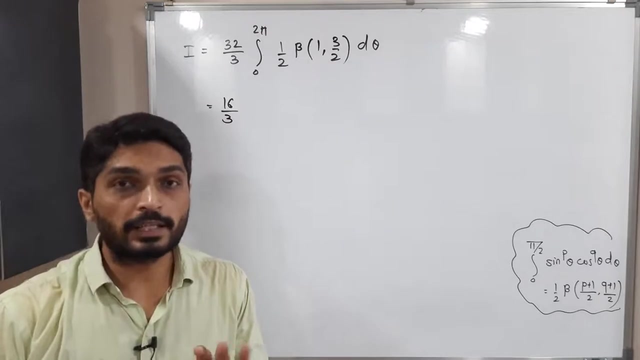 Okay, And yes, d theta, So let me remove this one. It is not required. Okay, So I am removing this. Yes, After that, 2, 2 will get cancelled. That means we will have 16 by 3.. So that beta 1, 3 by 2 will have some finite and constant value. 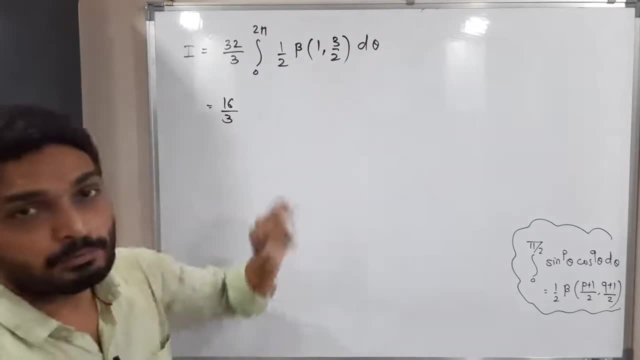 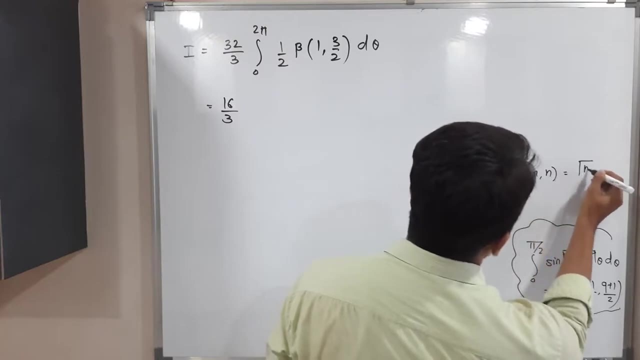 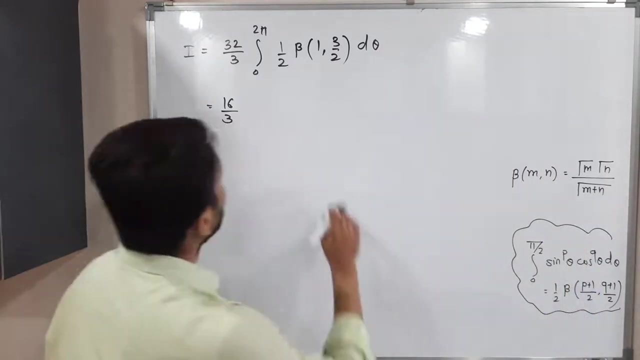 So we can take outside the integration integration. so you know the relation between beta and gamma function. let me write here: beta of m comma n is equal to gamma m, gamma n upon gamma m plus n. using this relation i'm going to find its value. so it will be: m is 1 and n is 3 by 2. so gamma 1, gamma 3 by 2. 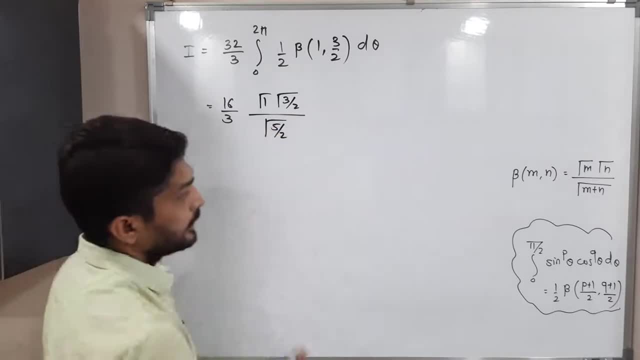 divided by gamma. 1 plus 3 by 2 means 5 by 2. see in denominator we add both numbers, so that's why it will be 5 by 2. integration of d theta will be theta having limit 0 to 2 pi. so this is equal to: 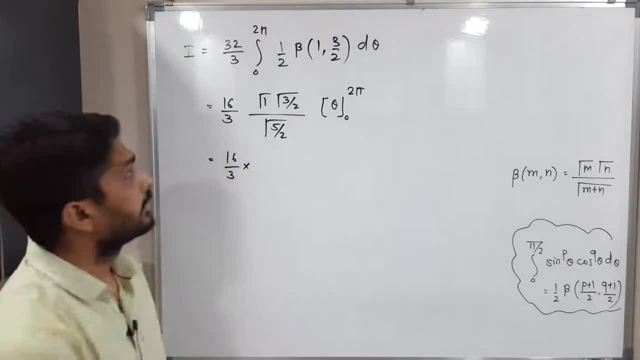 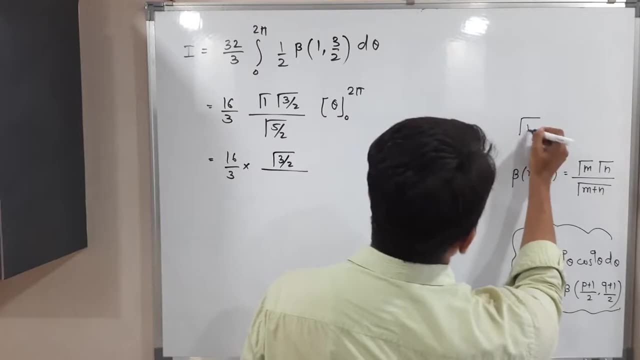 16 by 3. so you know that gamma 1 is 1, gamma 3 by 2, i will write as it is, gamma 5 by 2. so there is again one relation: gamma n is equal to n minus 1, gamma n minus 1. see this relation i'm going to. 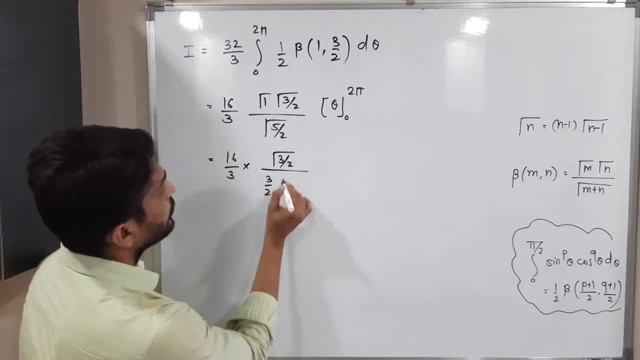 use of gamma function. so 5 by 2 minus 1, 3 by 2, gamma 3 by 2. so if you put upper limit, lower limit, we will get gamma 3 by 2. so if you put upper limit, lower limit, we will get gamma 3 by 2. so 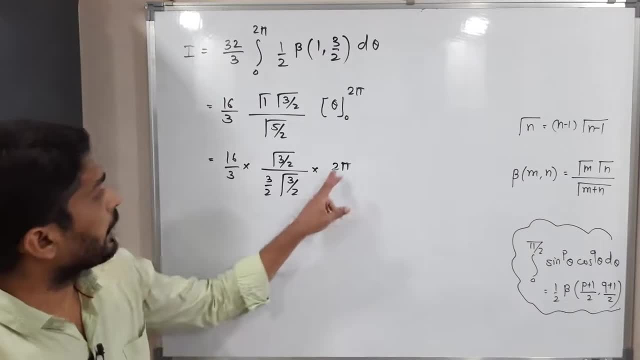 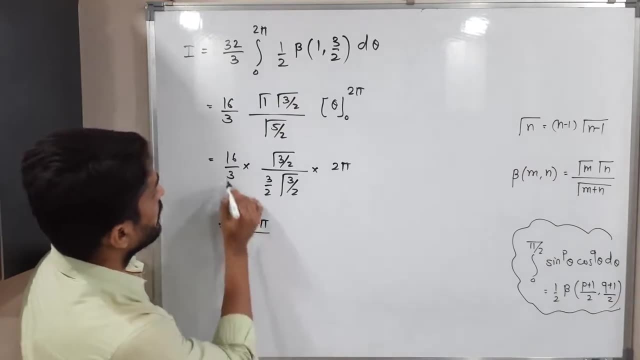 we will have value 2 pi, right? so what will happen? this 2 pi into 16, sorry, yes, so it will be 32 pi divided by 3 into 3, 9 by 2. we will have gamma 3 by 2. gamma 3 by 2 will get cancelled to each other.